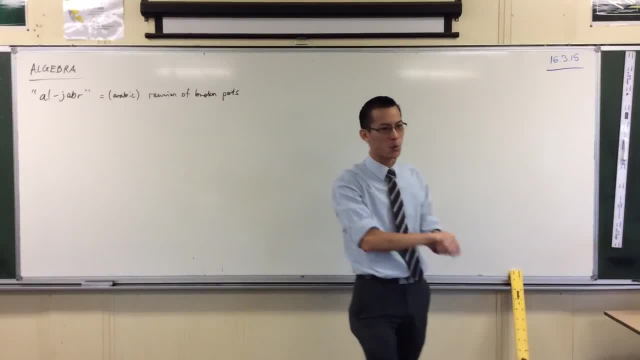 And it's the phrase used for setting bones after they are broken. right, They need to be reunited and put together. They're broken, but we can recombine them. Shh Now, as maths goes right. algebra is often experienced with a lot of difficulty, and there's a good reason for that, okay. 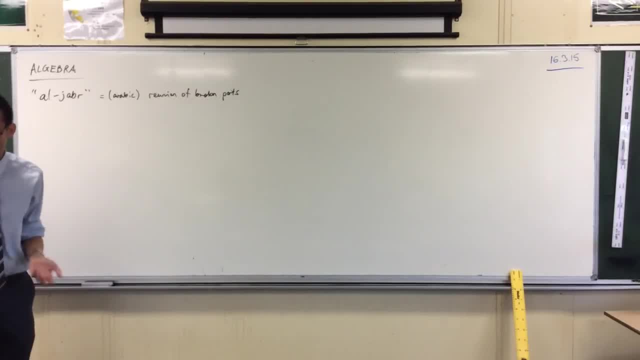 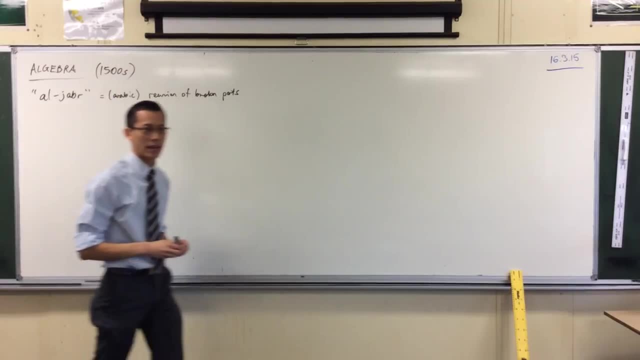 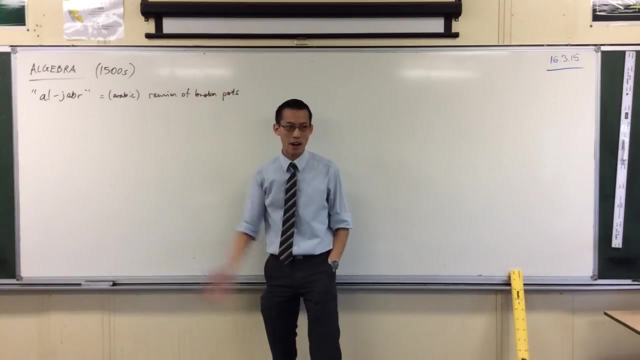 Algebra. well, compared to you guys, it's very, very old. It's very old. It's been around for hundreds of years. In fact, it's been around for about it's about 500 years, okay. But when you think about it on the mathematical scene, algebra is super, super nice. 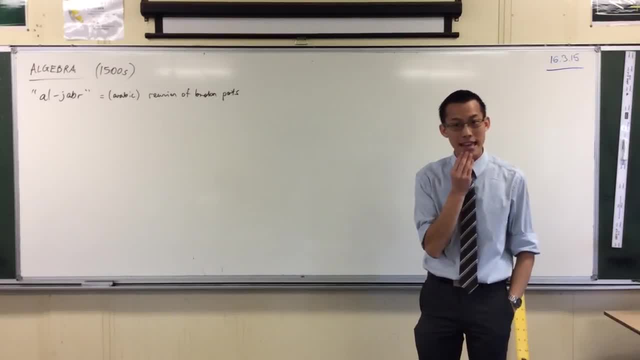 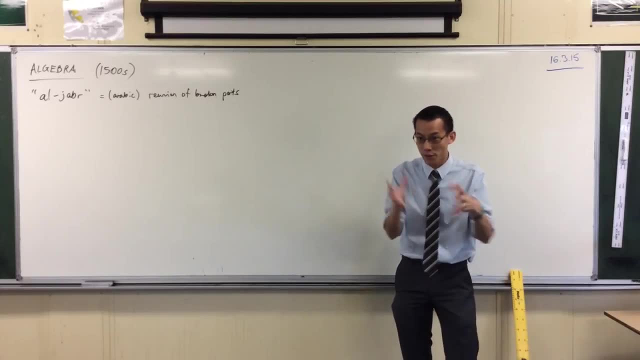 It's new. right. A lot of the maths that we've been learning is thousands of years old, because people have discovered it a long time ago. right, Pythagoras' theorem, for instance. right, We've learned that and civilizations have known about that for millennia. right. 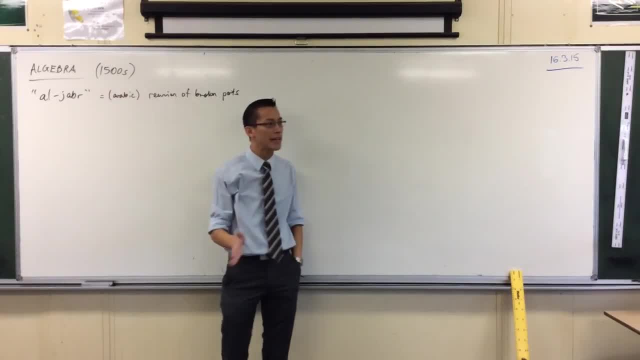 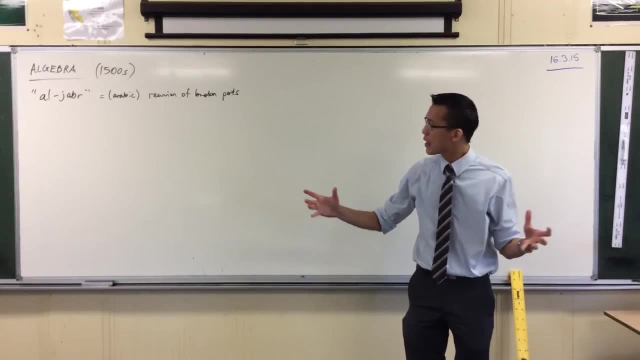 But algebra is new comparatively. It's only been hanging around for a few centuries Now, not just in terms of like society, right, But think about like the human race, If this has only been around for this amount of time. 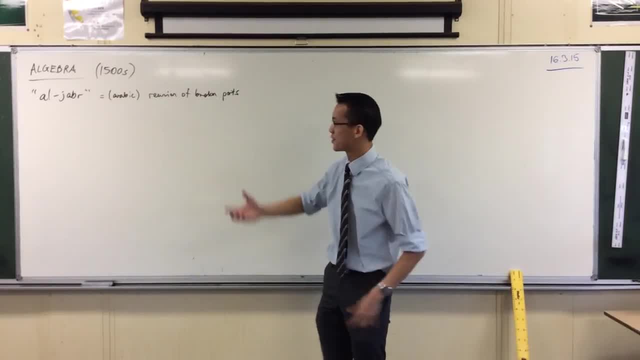 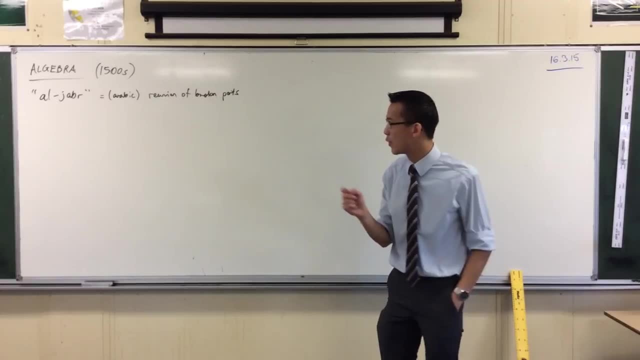 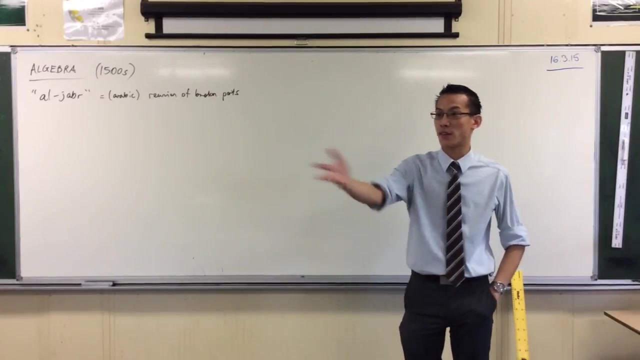 human brains haven't evolved to understand what algebra is. It's new, It's an invention, right, So it should make sense that we experience a little bit of difficulty when we get to this right. I have young children and one of the first things that you do, if any of you have younger siblings- 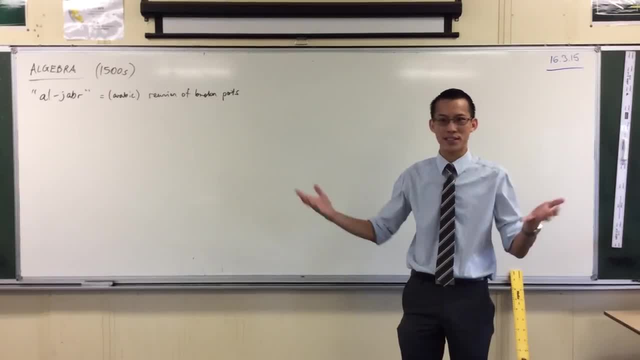 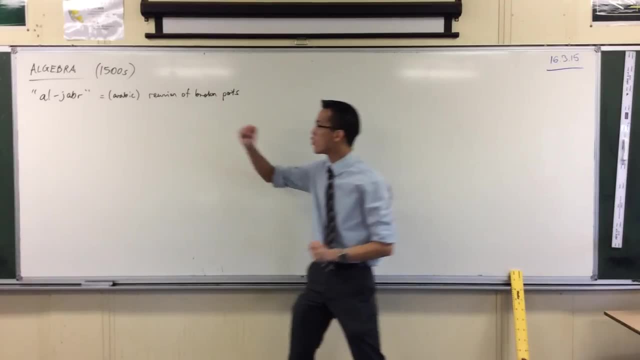 is you learn to count. Counting we have been doing since forever, right, Tens of thousands of years. We're very good at counting. Your brains are built for counting. Your brains are not built for this. This is not easy, right. 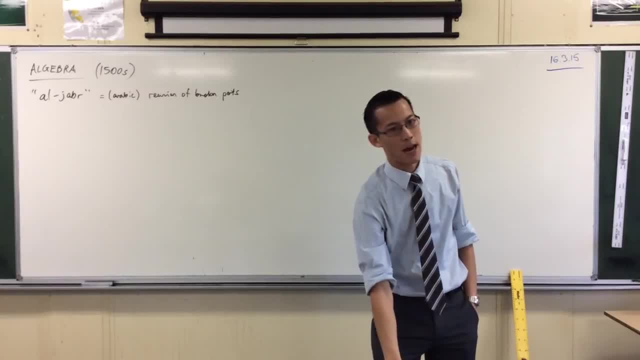 So we should expect a bit of a challenge. But even though our brains aren't built for this right- Perhaps, in fact, because they're not built for this- that's what makes this so powerful. In fact, in the 1500s- and you can write this down next to where your title is right- 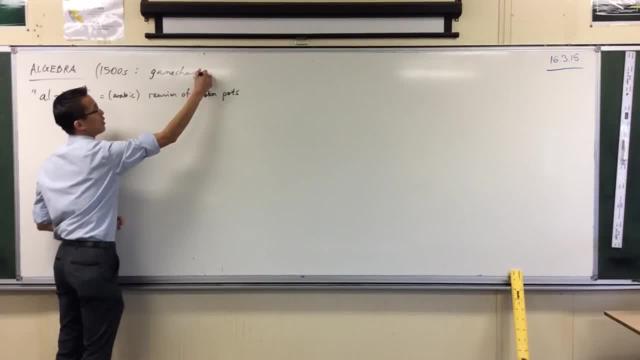 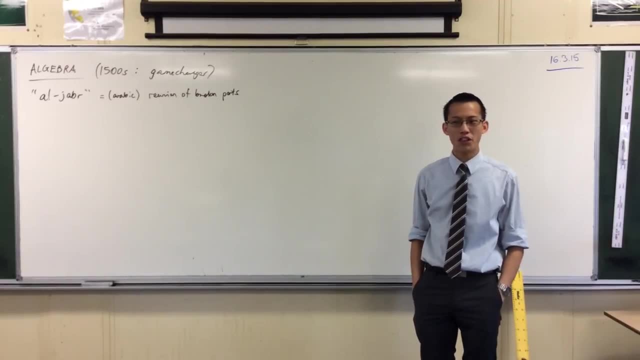 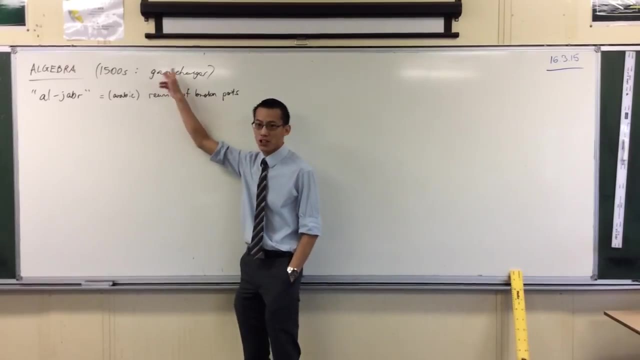 In the 1500s, algebra was what we call a game changer. It's a little bit like when someone invented gunpowder Right, Or the bow and arrow, And it changed warfare forever. Right, Algebra changed not just maths but problem solving. 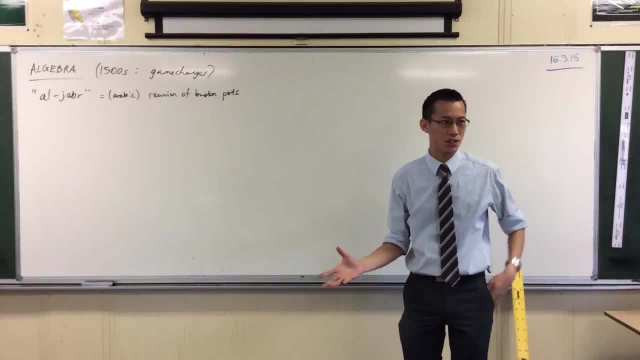 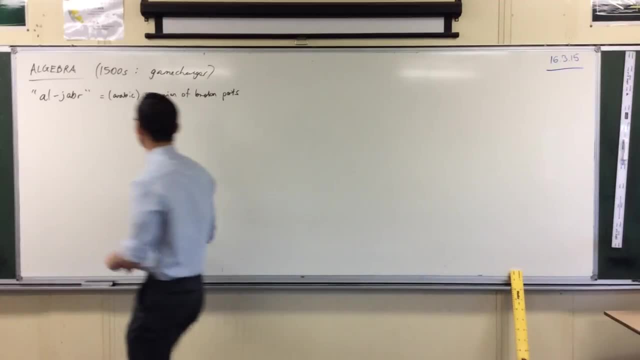 and the way that situations are approached and analysed. it changed all of those forever. Here's the key idea: right Yesterday I had a family lunch, okay, And for lunch I went to Costco and I bought. I bought some pizzas for lunch, okay. 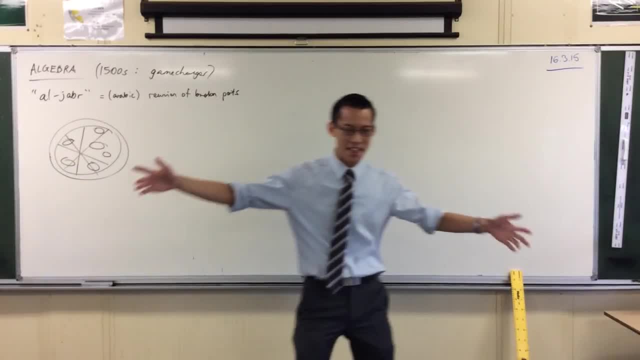 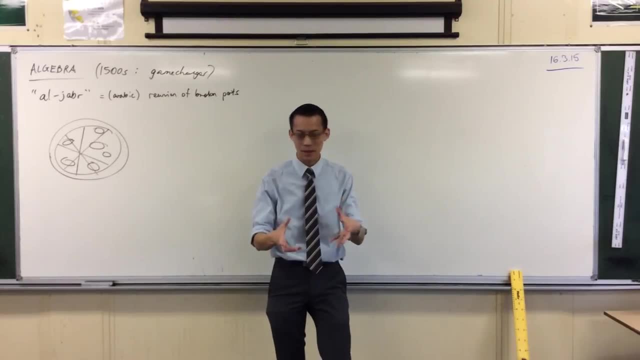 I bought some pizzas for lunch. They're ridiculous things. They're so big you can't fit them in a standard size oven. okay, I had to slice it into pieces and pop it in to warm it up. They're enormous things. I could barely fit it in my car. 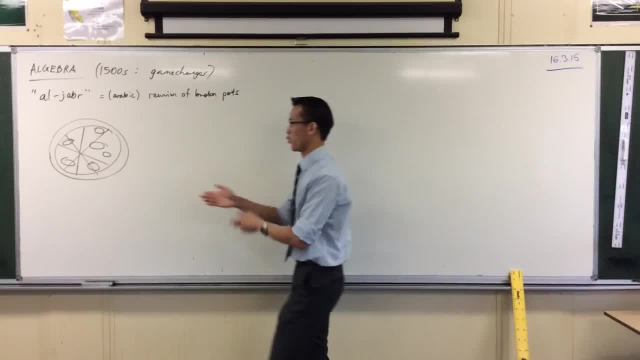 I bought two because I'm a big family And they're all sliced into. Actually, this is wrong. They're sliced into six slices And these are enormous pizzas, right? So when they're only six slices, one slice is literally like the size of a plate. okay. 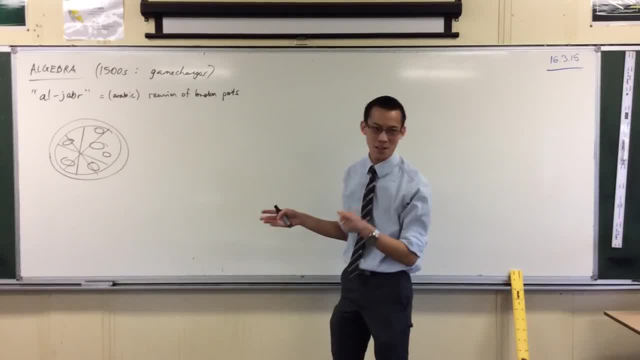 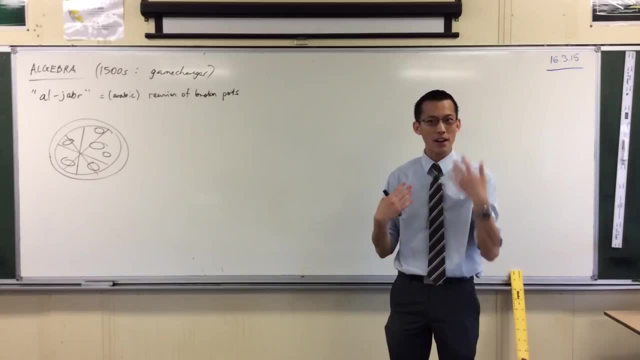 So it's like: okay, here's your one slice. okay, Now here's what we did. I told you I had two pizzas, So I had 12 slices of pizza, 12 slices. And then I wanted to know well how many slices of pizza. 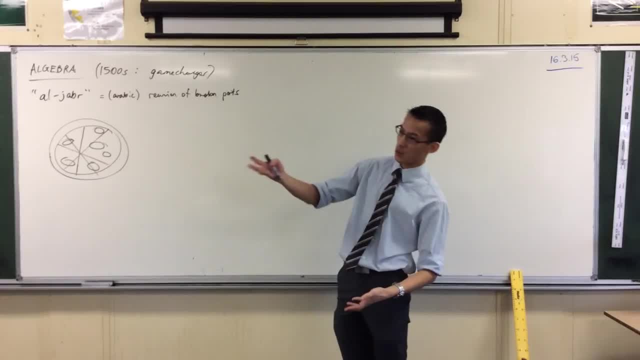 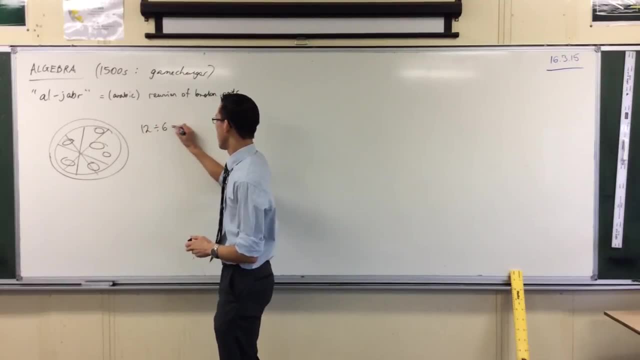 could each person have, And there were six adults there, so I was like: 12 divided by 6, okay, Everyone could have two pieces easy, okay. 12 divided by 6 equals 2, okay. Now, these are what maths people do. 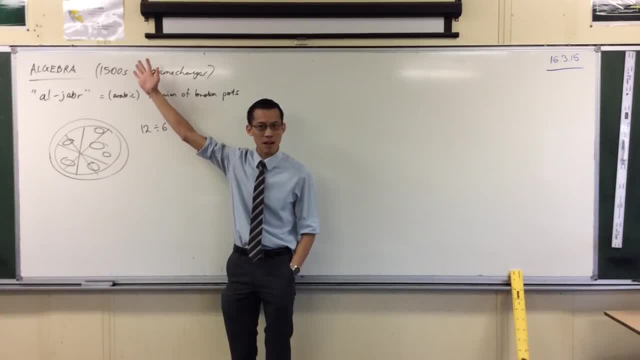 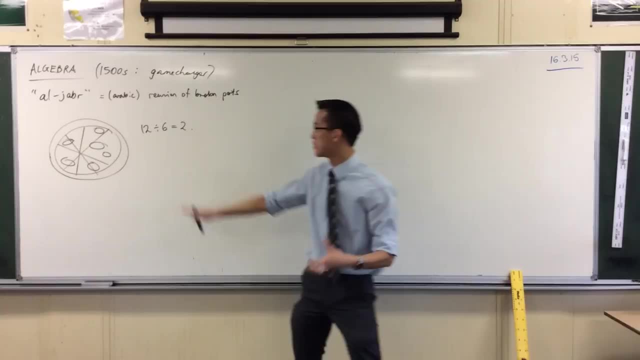 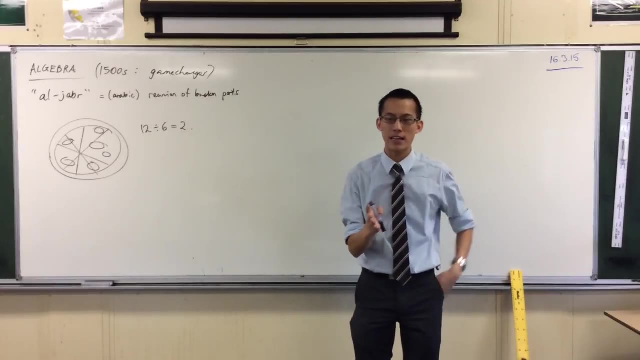 This is what maths problems were like for centuries, right? They're problems where you know what everything is equal to and you have a problem and you can work with those numbers and you can come up with an answer. okay, Algebra is a game changer because it's where people realise. 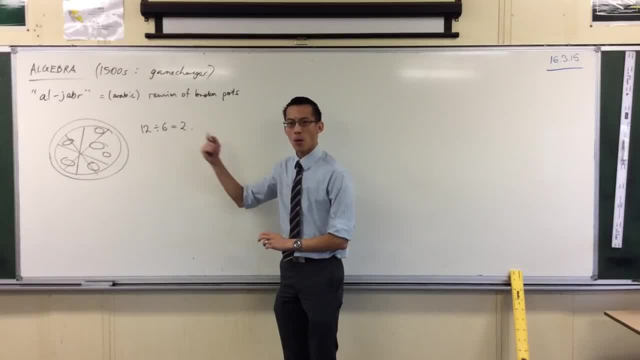 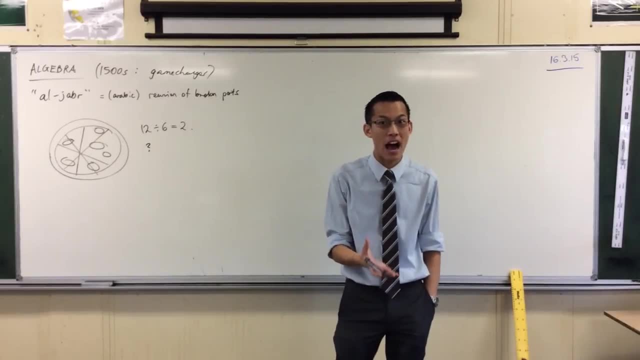 wait a second. you can have a problem where you don't know what the numbers are, where you can like I don't know how many pieces of pizza maybe. I want to know how many pieces of pizza I should buy, right? 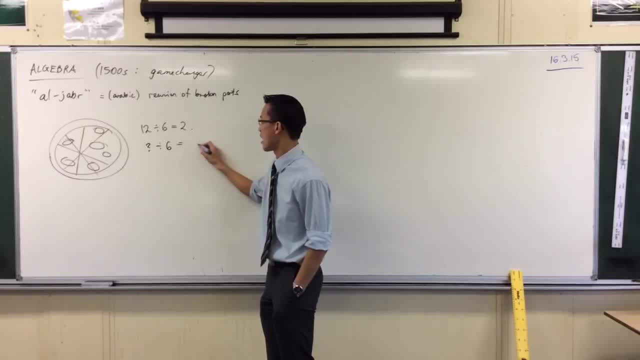 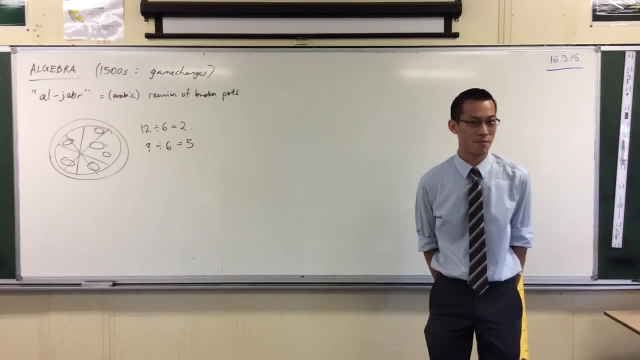 And I know that I'm going to have to divide it by 6, and then I want say: I want, you know, 5 slices for everyone, because it's going to be some very hungry people, or something like that, right. 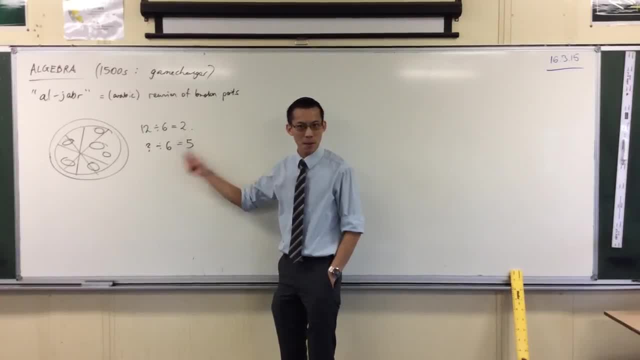 It's this idea that you cannot know what the numbers are Like. maybe I don't know how many pizzas there are, and maybe I don't even know how many slices they're going to be sliced into, But if I want something, I can still work with these numbers. 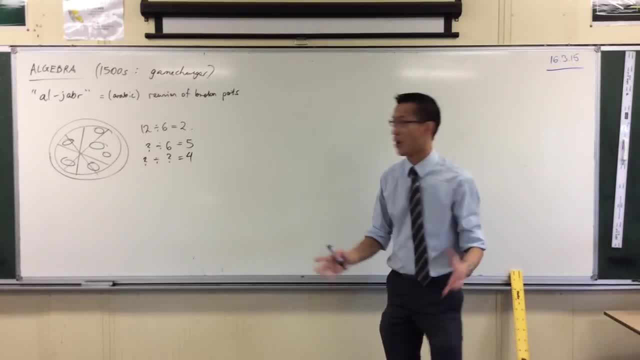 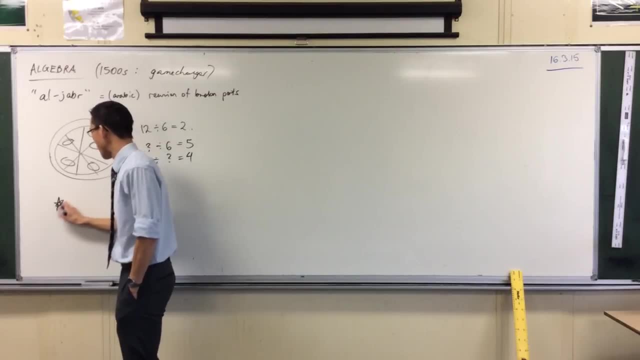 even though I don't know what they're equal to. That's the game-changing idea. That's the idea behind algebra. OK, Which is why in algebra- and this is a little subheading you can make- the key idea is that of a. 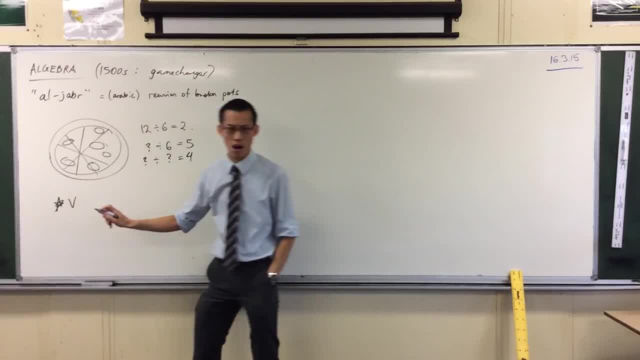 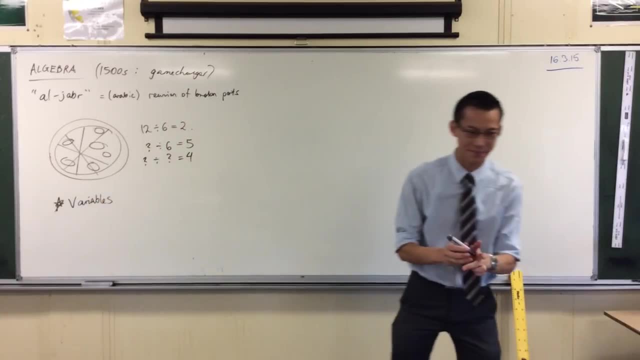 Starts with a V. Does anyone remember what the word is in algebra? They're called Variables, Variables- OK, so write that down. That's how many Question: Why do we have algebra, if it just makes it a bit harder? 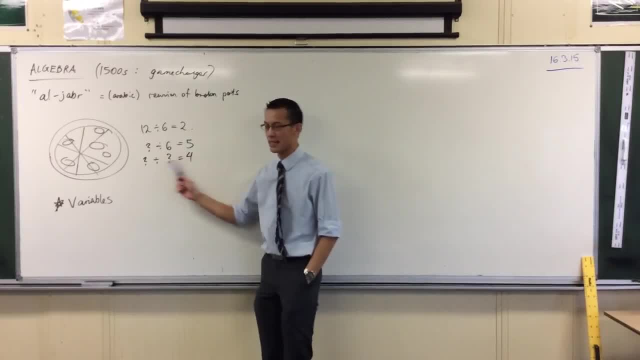 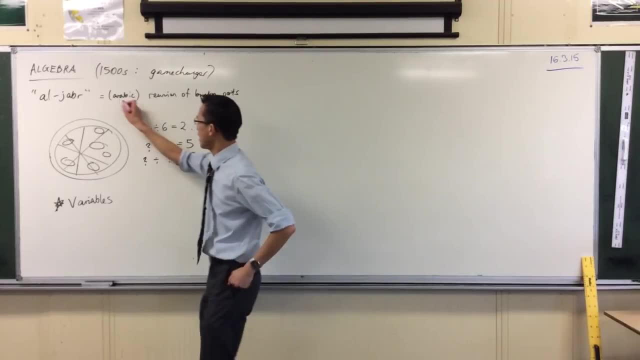 OK, Does it help? Yeah, sure. So let me come to this idea: Why do we have algebra if it's so hard? OK, Maybe this is a good opportunity for me to explain. Algebra's a bit weird in that it's an Arabic word. 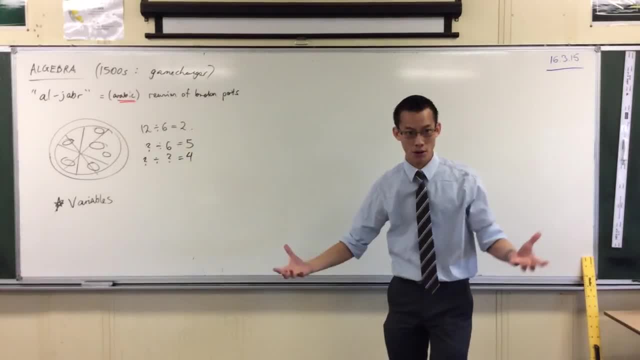 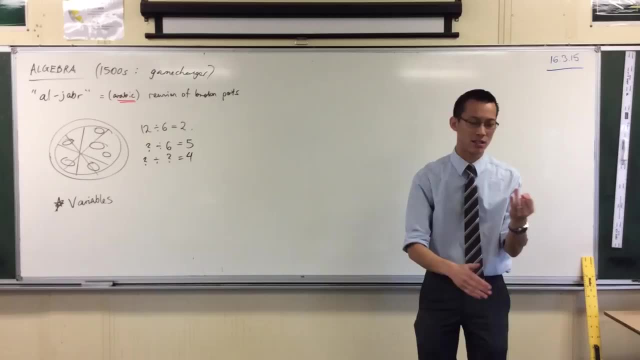 The reason why is if you think about all of the other words you know and how we learn things right, Think of all the words like attached to subjects like geography or mathematics, or even within mathematics, like geometry and trigonometry and all that kind of thing. 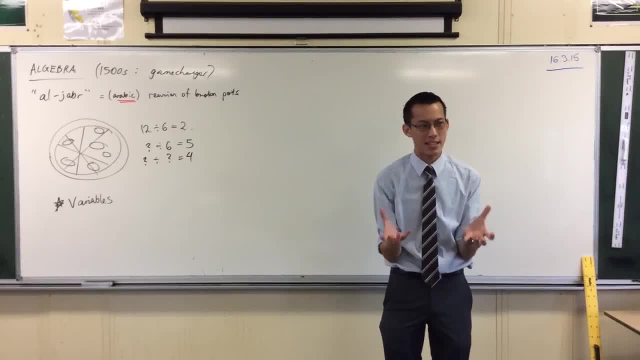 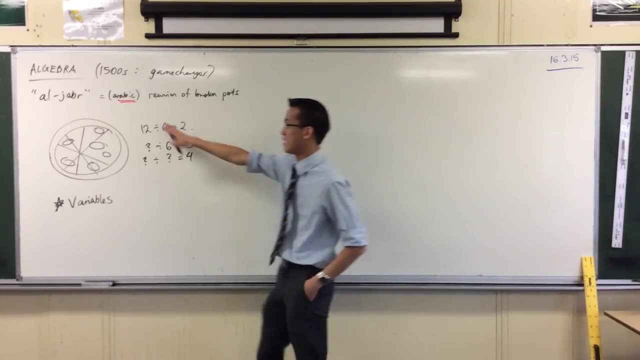 All these words, all these words, they all come from Latin. Now maybe you're like, You're sorry, Lots of things come from Latin. That makes sense because, as society, Western society, was growing up, all the people who were like scholars, 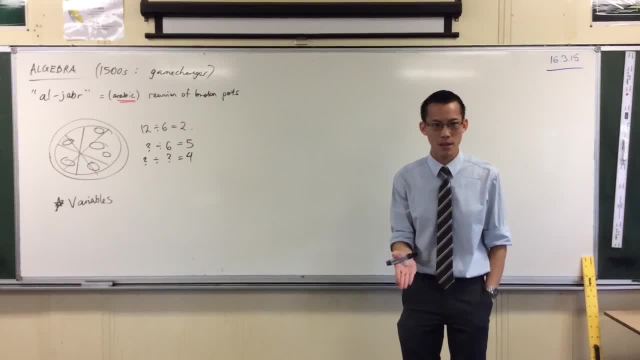 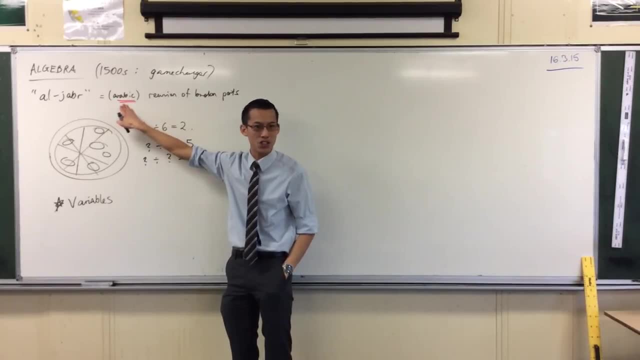 and people who went to school and learned. they all learned in Latin, So it makes sense that all of our learning words and school words come from Latin. OK, But this guy comes from another language. entirely right, It's because for centuries we weren't doing maths like this. 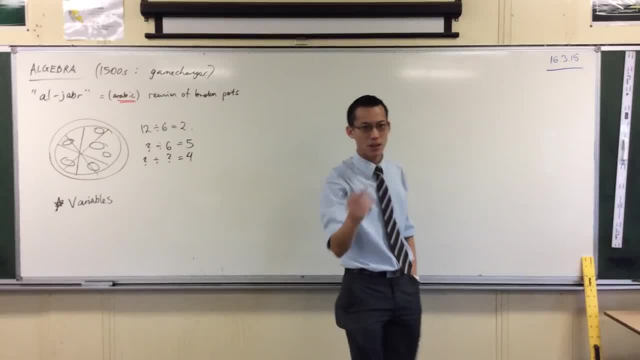 But we saw that these guys were and like a game changer does. it doesn't necessarily mean that. it doesn't necessarily make things harder. It opens up a whole bunch of harder problems that you couldn't touch at all unless you knew this right. 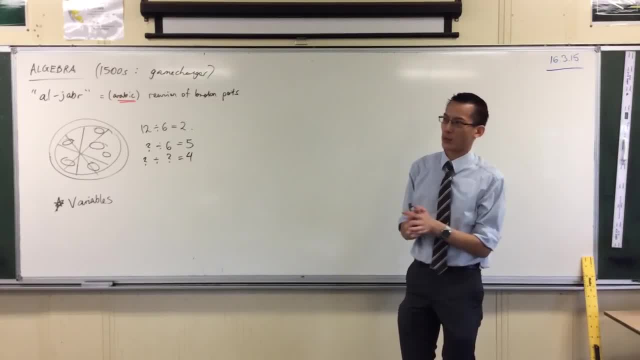 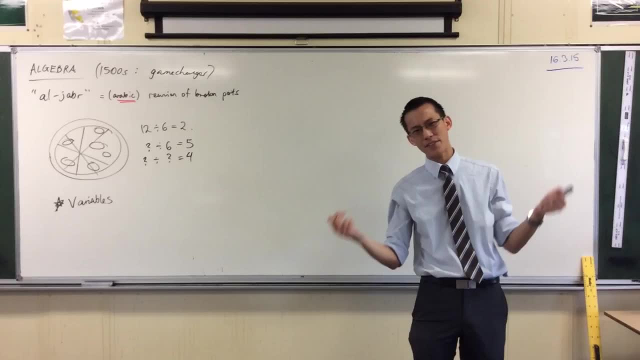 So the reason why algebra is harder is because it's a little bit like: well, it's a little bit like the way driving- driving is harder than walking. It's like: why do I have to learn driving? Well, because you can go all these different places. 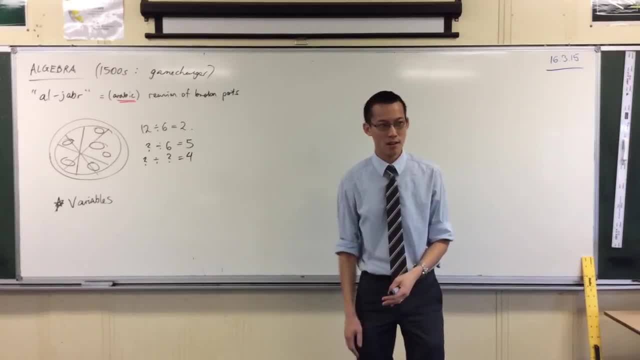 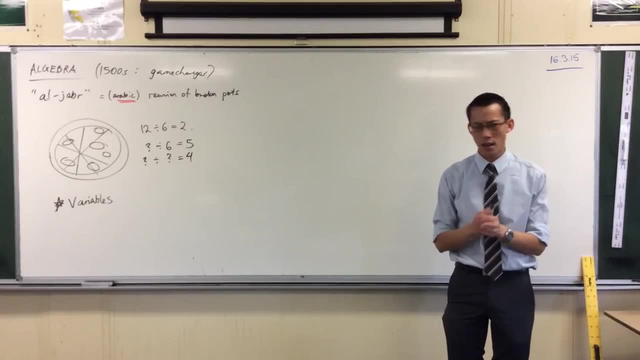 if you can drive But you can't go if you can walk And in the same way, flying a plane is harder than driving a car, because flying a plane can take you all these different places that driving a car can't. Does that answer your question? 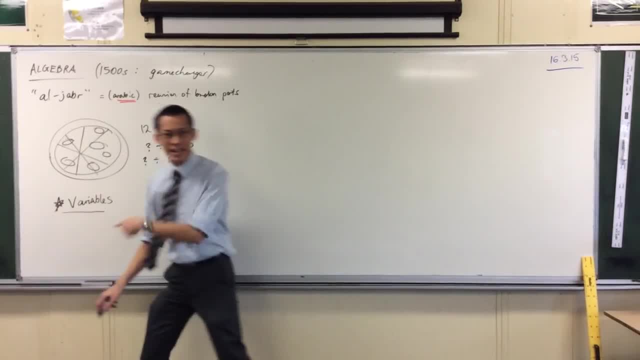 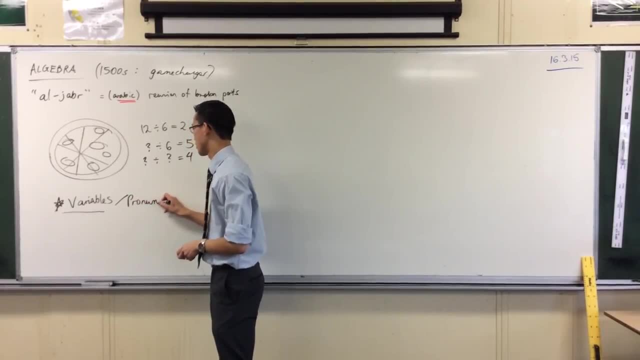 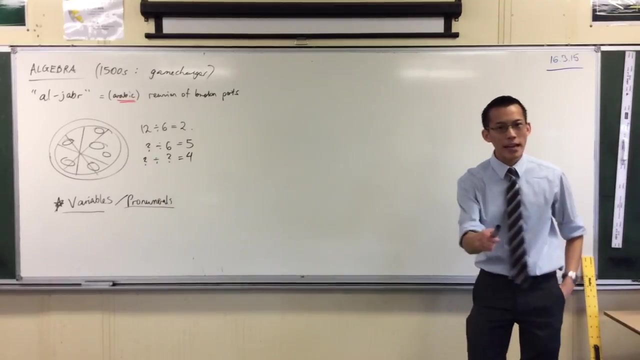 OK, So the heading you made was variables, and next to that you can put another name for the same thing, which is pronumerals. You might remember that Pronumerals. So this whole idea of algebra is solving problems where you don't know what the numbers are. 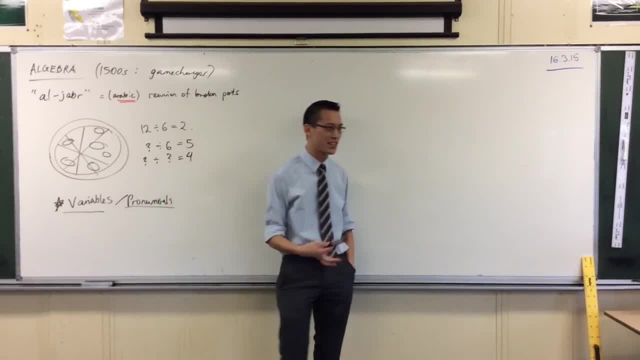 Right. But you can see it starts to get tiresome if every time you don't know what a number is, you write a question mark, Right? We've got different numbers that we don't know what they are, So I need to be able to distinguish between them. 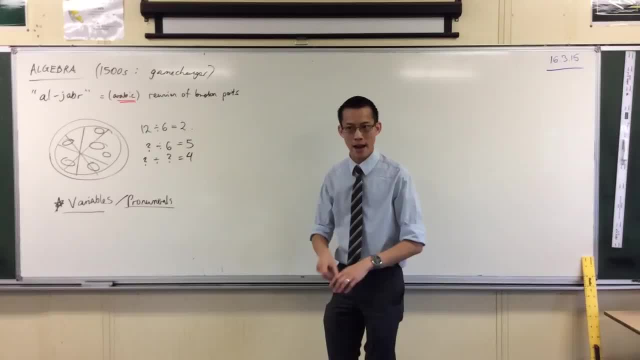 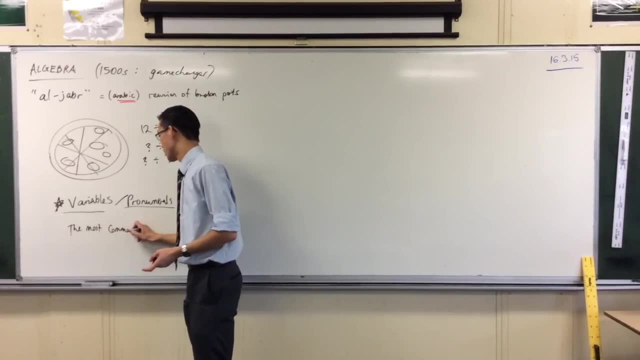 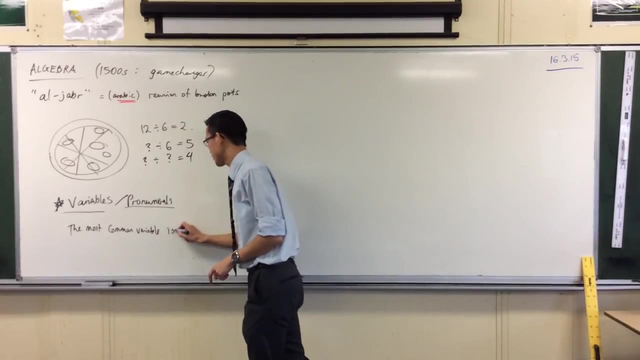 And that's what pronumerals and variables are about. OK, So, for example, you know, the most common variable is x. Very good, Now I'll tell you another story another time about why it's x. OK, But it's why we have things. 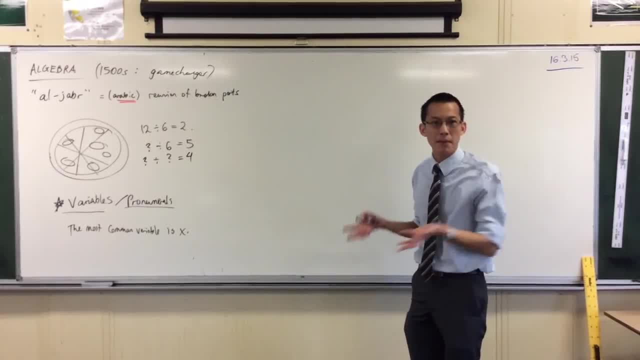 you know, it basically means unknown, Like it's something, but I don't know what it is, Which is why, by the way, just as a side note, it's why x-rays are called x-rays, Because when they were discovered, 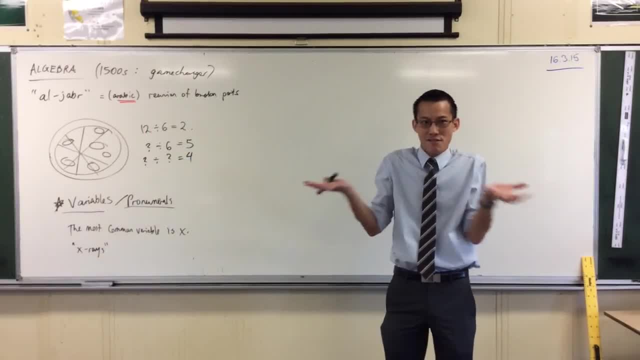 they were a kind of radiation and they were like: I don't know, It's a kind of radiation, but we don't know anything about it. It's not visible, it's not infrared, it's not UV, It's something else. 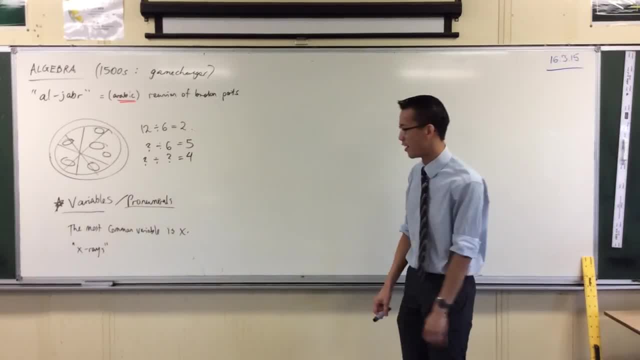 Unknown, So they called them x-rays and then the name just kind of stuck, even after we found out what they really are. Where are they? OK, You can go to your science class and ask for that, OK, Simple idea, Right. 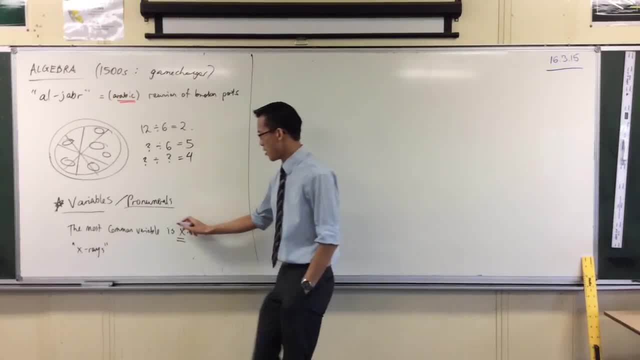 If we say x is some kind of number, right, we call it a variable because well, it can change, Right, Just like the number of pizzas you buy it can change, It can vary. So it's variable, Right. 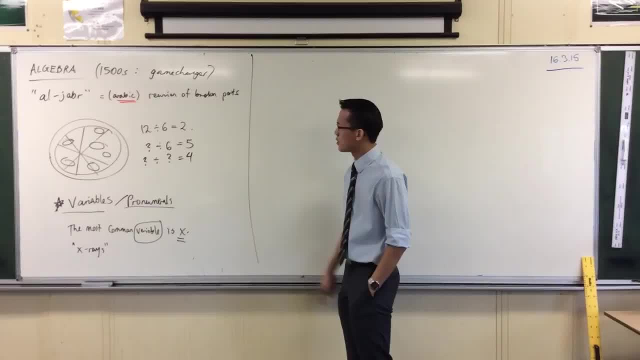 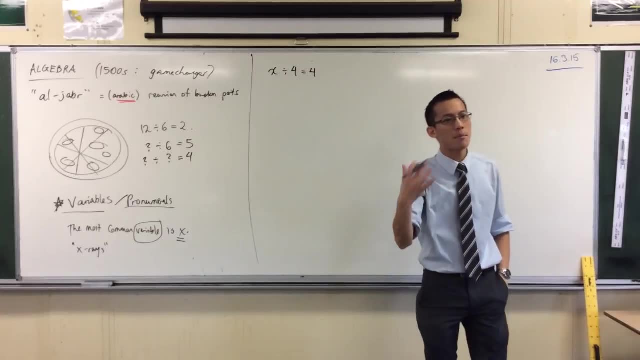 We use the pronoun real x to stand for that. OK, So we could write, for instance: x divided by 4 equals 4.. Right, So there's some number in this case. right that, if I stick it in here, 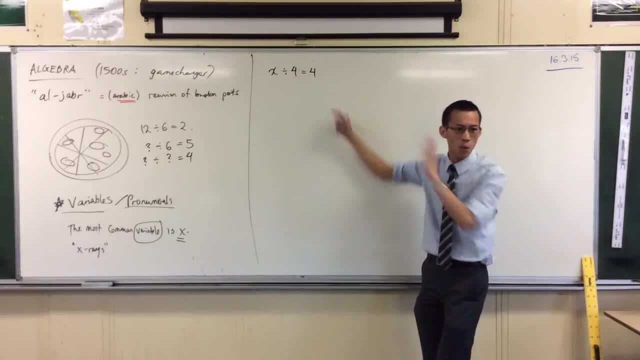 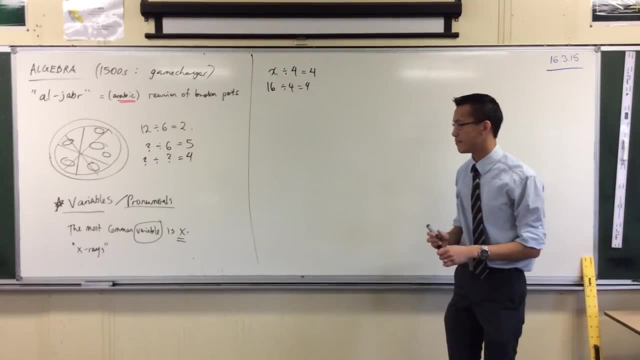 it'll equal 4.. And that's called solving this equation. What is the number you divide by 4?? It's 16.. It's 16.. Very good, Brandon, Sir um, before x? um, you wrote a different way. 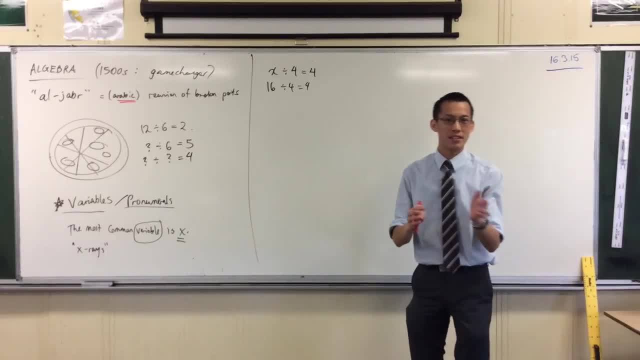 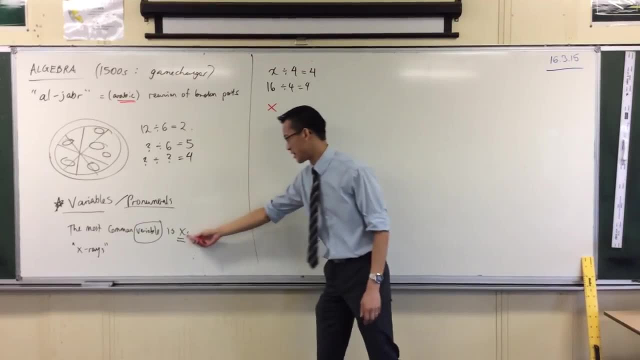 Oh yeah, sure, OK, That's a good thing to mention. So there's lots of ways to write x Like you might write an x like this. I'm going to encourage you, even though I did it there. 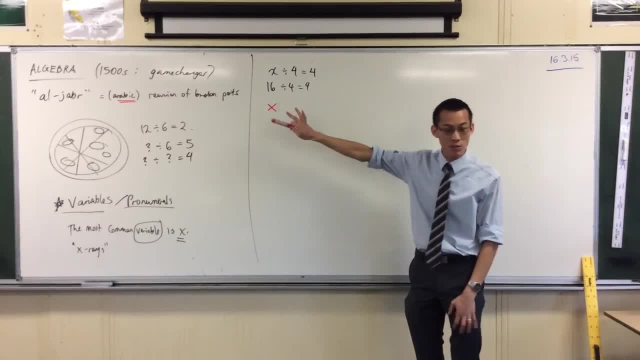 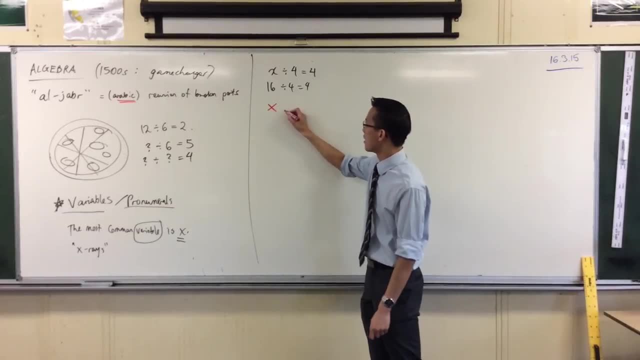 um, I'm going to discourage you from writing x like that, And the reason why is because that looks exactly the same as a multiplication sign: right Times times, So that's exactly right. So I think, um, um, this is. 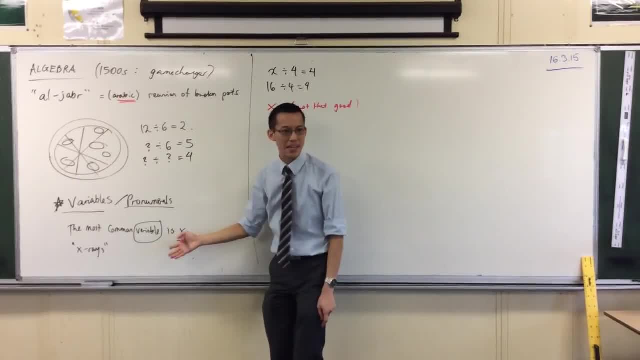 this is not that good. I mean, if you have a look down there right, you can see it's kind of unambiguous what I mean here, which is why I can kind of get away with it. But when we write equations and expressions and so on, 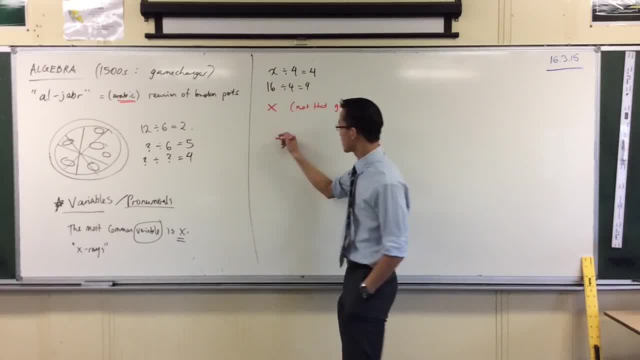 it's probably better not to write it like this. Here are my suggestions. Um, you could write it like this: That's kind of like a C and a backward C next to each other. Or, alternatively, you could write it like this: 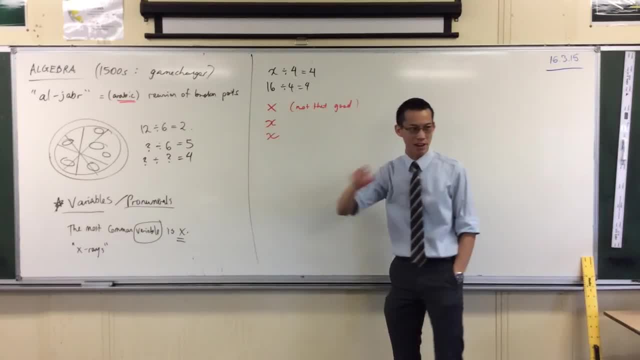 You could write it with like a kind of wiggly, like a multiplication sign, but one of the signs has like kind of tails next to it. Uh, kind of. So I I think these are these are better. You'd be able to tell them apart. 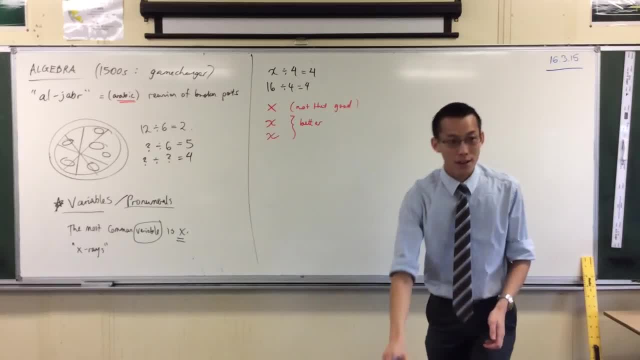 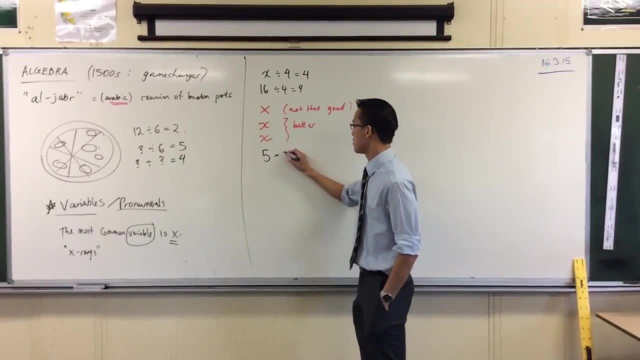 Okay. So, if you remember, there's a bit of shorthand you can use. For example, instead of saying 5 times x, we tend to write that just as 5 x, Right? So you can write it like this: 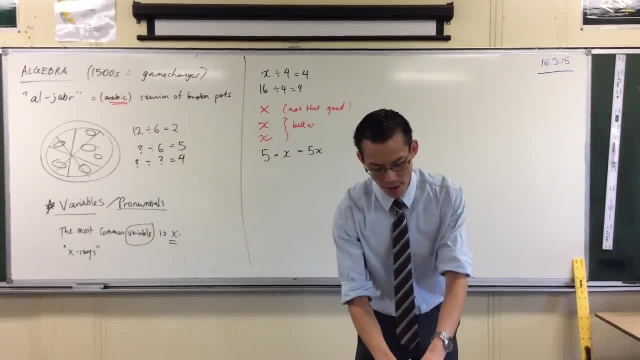 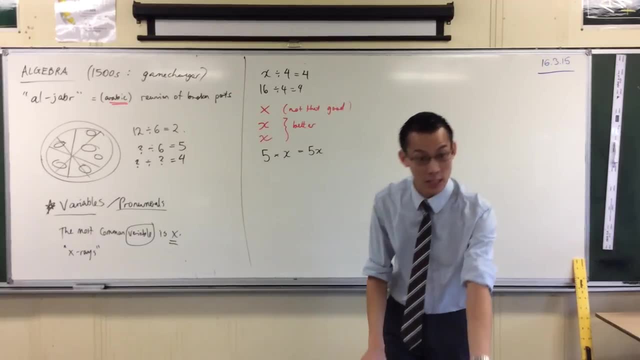 So rather than saying, for example, you know, uh, 5,, 5,, 5 boxes of pizza, You could just say 5 pizzas. Right, It's the same kind of contraction, just making things faster. So the answer of it is: 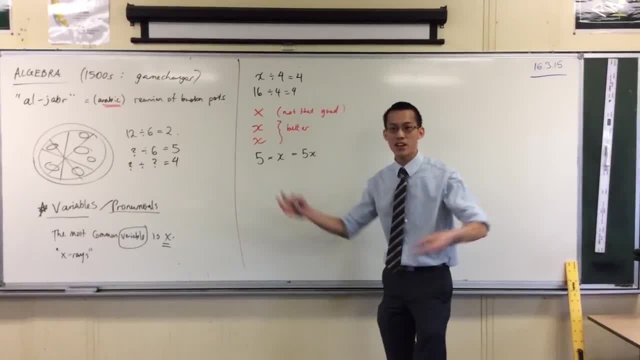 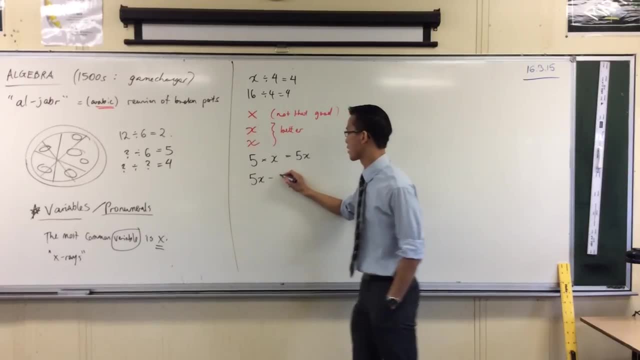 basically just take out the equation: Yeah, that's right, It's, it's not that hard, Okay, Um, now you can combine all kinds of other operations, and order of operations is still the same. So, for example, if I showed you this: 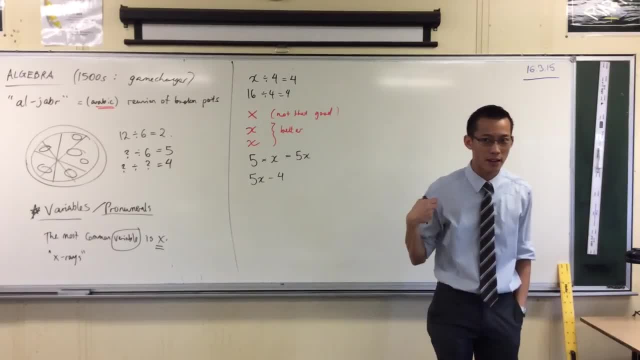 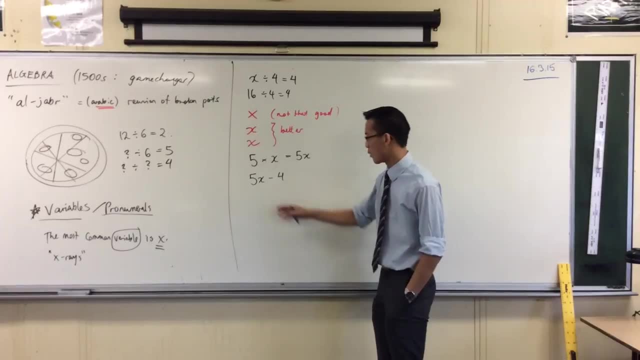 5. x is 5 times x, Right, So what kind of operation would you do? first Think about it carefully. Yeah, Tendai, Would you want to find out what x is? so you do the minus first, Okay,